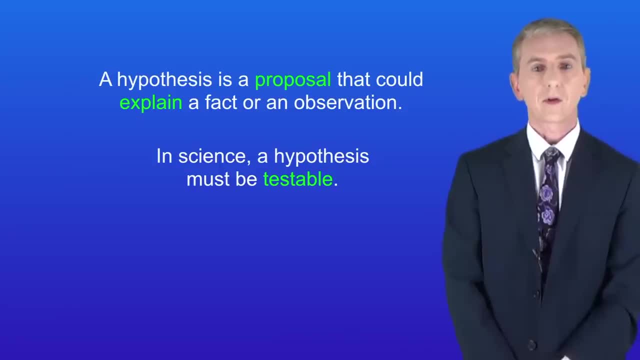 Okay, so we're going to start by looking at an experiment called the disappearing cross reaction. We're going to use this to explore the effect of concentration on the rate of a reaction. If we react sodium thiosulfate solution with hydrochloric acid, then one of the 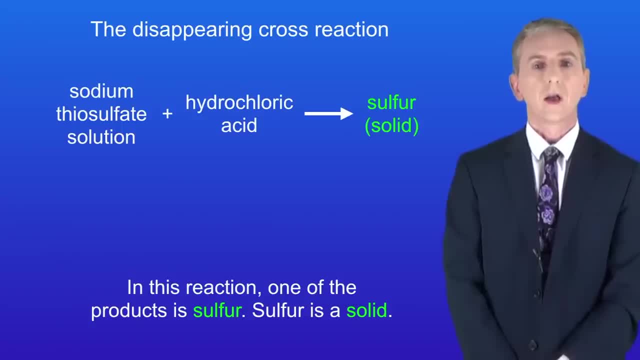 products is sulfur, and sulfur is a solid. The sulfur makes a solution go cloudy. Scientists call this cloudiness turbidity. We can use this to see how long the reaction takes to finish. So let's take a look at the method First. we 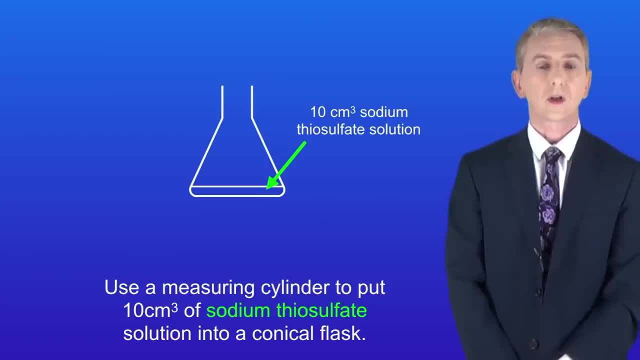 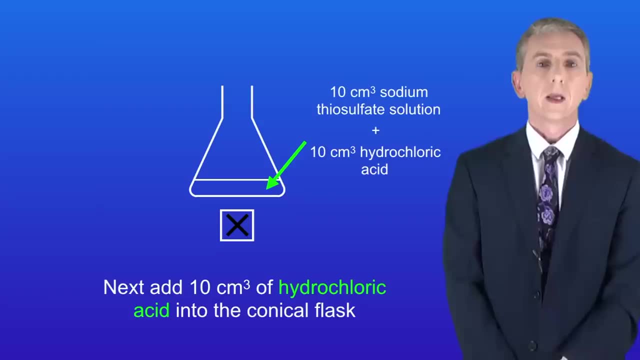 use a measuring cylinder to put 10 centimeters cubed of sodium thiosulfate solution into a conical flask. We then place the conical flask onto a printed black cross. Next, we add 10 centimeters cubed of hydrochloric. 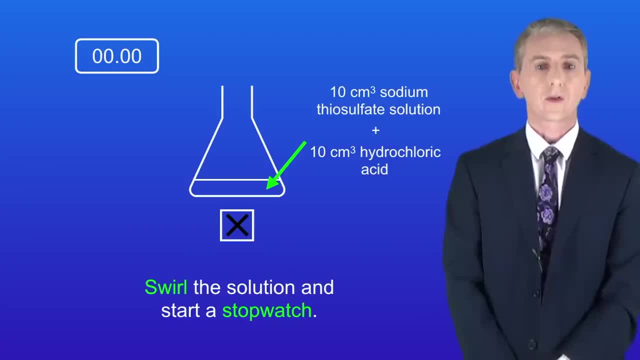 acid into the conical flask. Now we swirl the solution and start a stopwatch. We now look down through the top of the flask. After a certain time the solution will turn cloudy. We stop the clock when we can no longer see the cross. We then 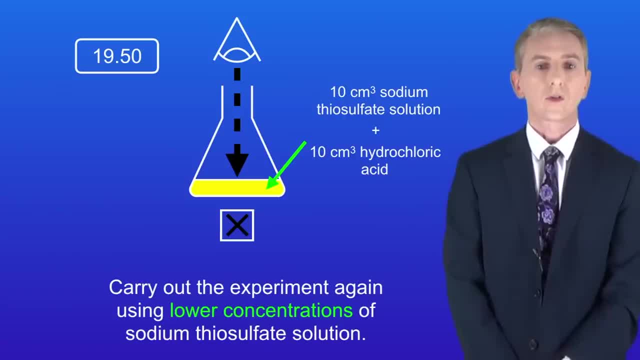 carry out the experiment again using lower concentrations of sodium thiosulfate solution. Finally, we repeat the whole experiment and calculate mean values for each concentration of sodium thiosulfate solution. Remember that we do not include any anomalous results when calculating a mean. Now there is one important idea linked to this practical, which you need. 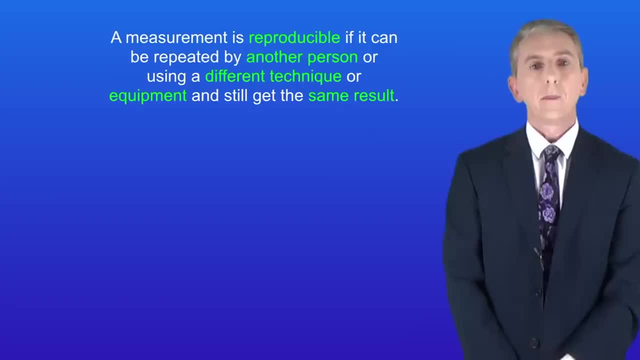 to learn, and that is reproducibility. A measurement is reproducible if it can be repeated by another person or using a different technique or equipment, and still get the same result. Now, the problem with the disappearing cross experiment is that different people have different eye sights. That means that 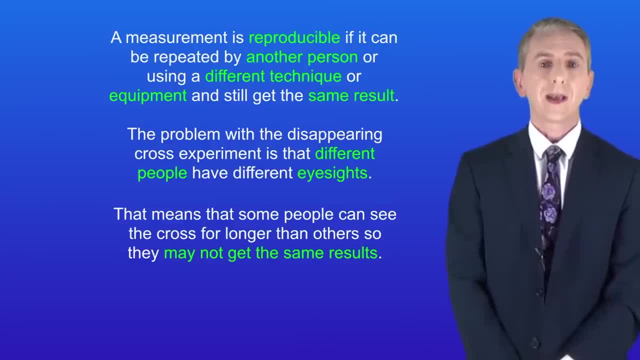 some people can get the same result. The problem with the disappearing cross experiment is that different people have different eye sights. That means that some people can see the cross for longer than others, so they may not get the same results. However, because all the students use the same size printed cross, hopefully this problem won't be too great. 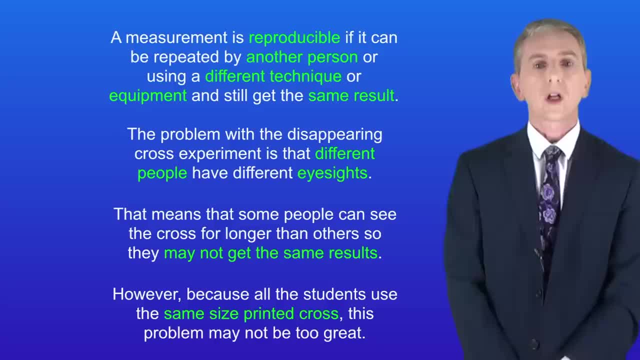 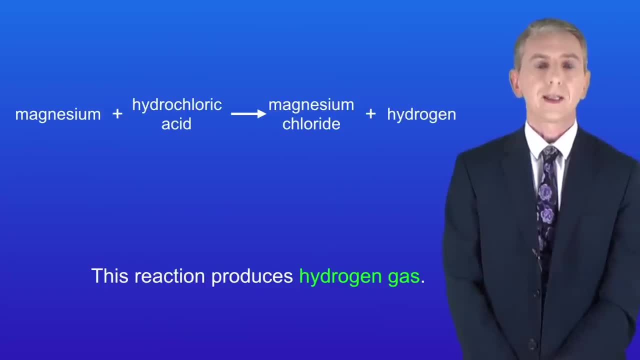 Okay, we're going to look now at the second method for this required: practical. We're going to measure the volume of a gas produced by a reaction. Take a look at this reaction. Here we're reacting magnesium with hydrochloric acid. This reaction produces hydrogen gas, and this allows us to measure.